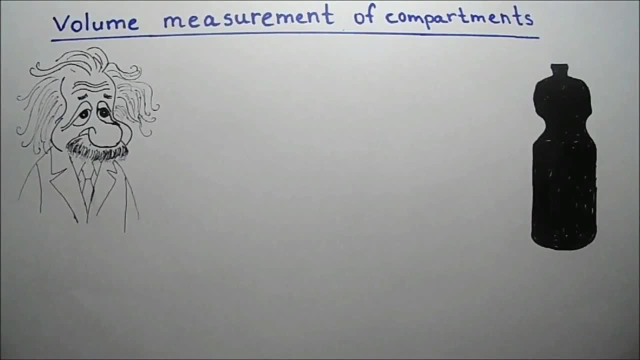 open and see how much water is there- right. But how do we know that 60% of total body weight is water? We don't have any lid to open and see how much water is inside your body, right. But the good news is that we have the formula and brain to calculate it. even though we can estimate both, 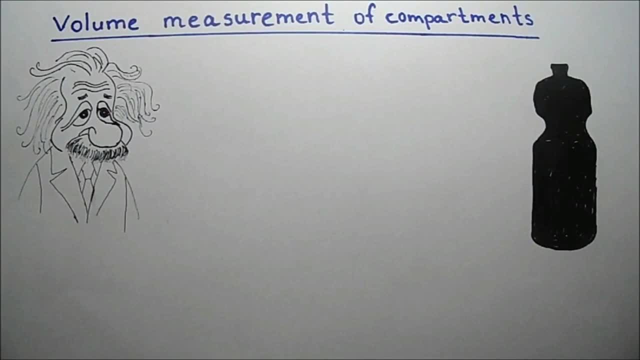 your intracellular and extracellular fluid compartment. Let me assume that you have not the patient's anthropometric measures and you have to estimate the water content inside the bottle. Let me assume that you have not the patient's anthropometric measures and you have to estimate the volume of the extracellular fluid of the. 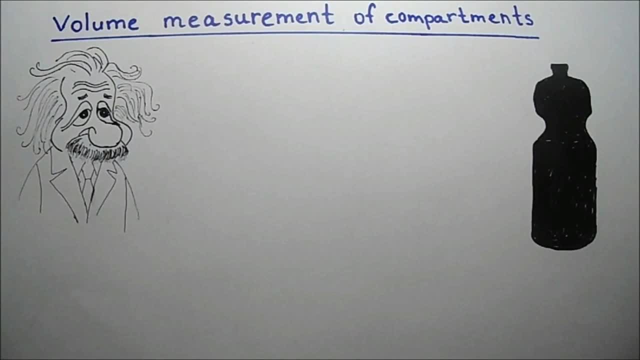 patient To make it clear. I mean the concept of measuring of volume compartment. let's imagine you cannot open the black bottle and you need to estimate how much water is there. So we can do it without opening the bottle. but we need something more. We need any tracer and the 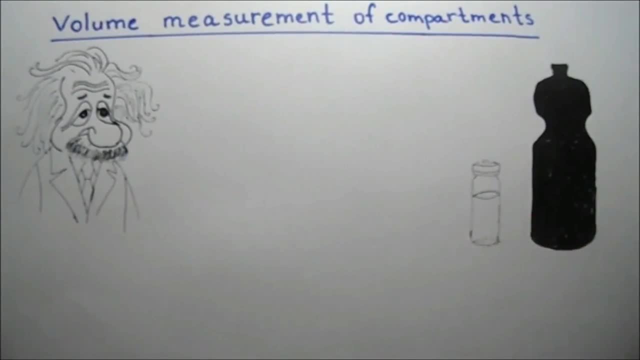 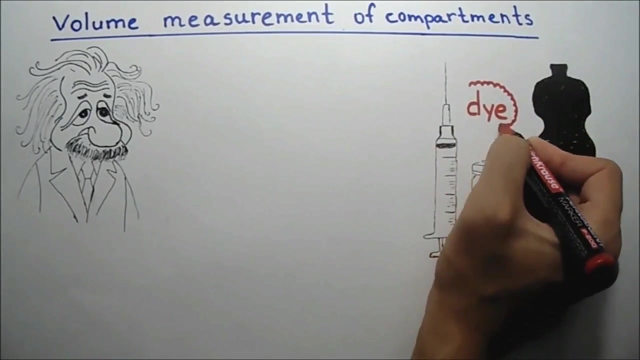 tracer- substance must be easily diluted in the water- and a syringe to add the tracer into the plastic bottle. And, of course, our magic formula which I've talked about. So we will use a dye, because this tracer dissolves readily in the water. Let's suppose that you have added 10 mg of dye. 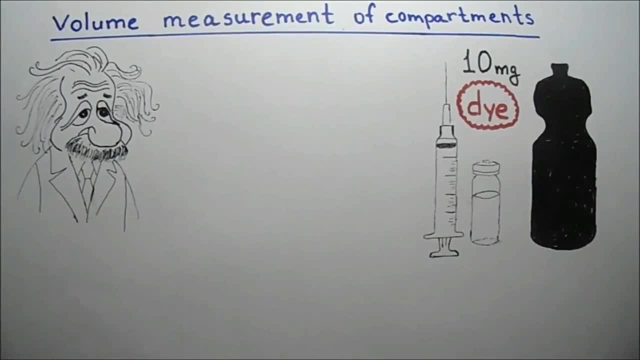 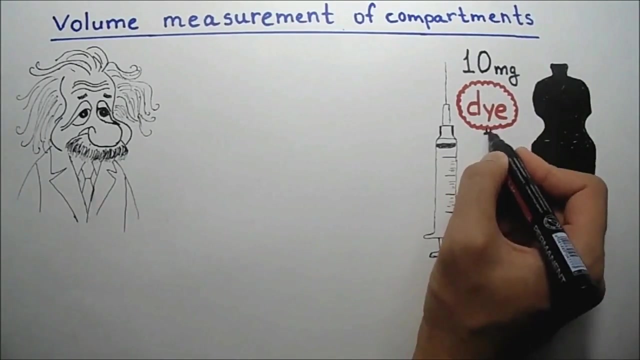 After that you have to shake the bottle well to dilute our substance. well, Then we will take some amount of the fluid back to the syringe and estimate the concentration of dye per milliliter of the water. Now let's suppose that the concentration of our tracer is 0.01 mg per milliliter, and now we need the 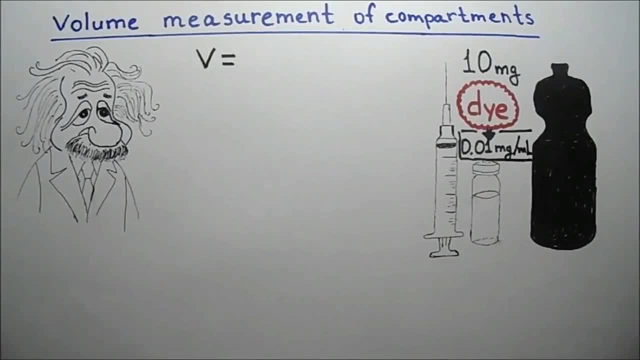 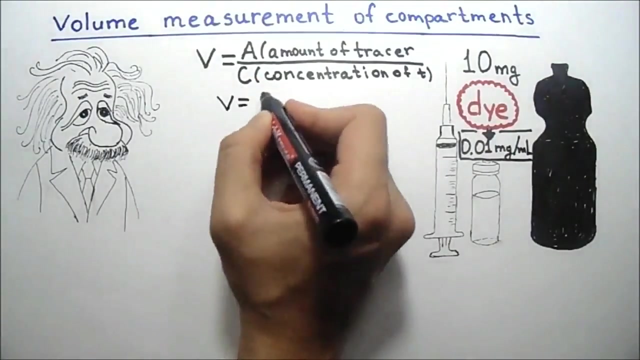 formula which I've talked about. This formula says that the volume of the compartment is equal to the amount of tracer which I've added right now, divided by the concentration of the tracer in the compartment. So we write these points just to remember Now what we have here. We have our tracer. 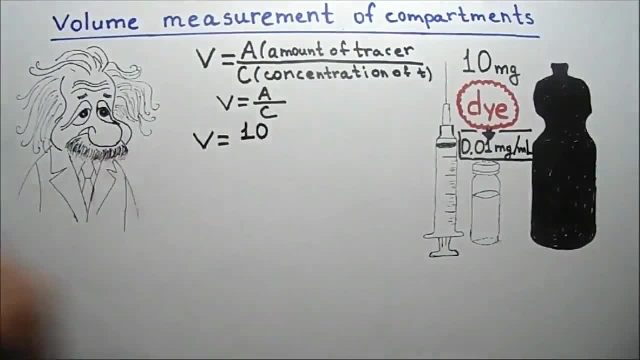 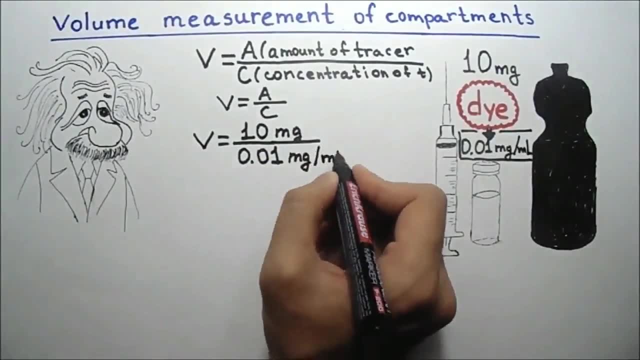 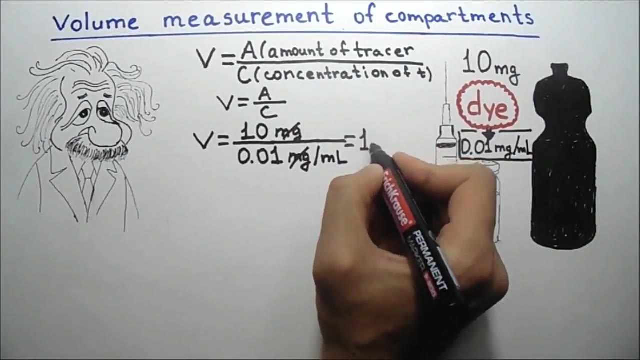 which I've added is 10 milligrams and the concentration of the tracer which we have got after the dye has been diluted. It is 0.01 milligram per milliliter. So 10 divided by 0.01 equals 1000 milliliters, So we have a liter of water inside the bottle. The same thing is with 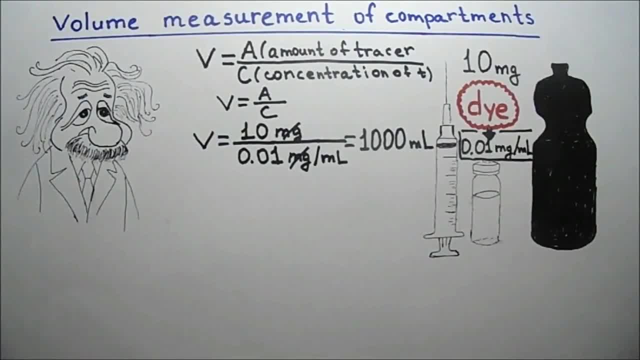 our body fluid compartments. So let's figure out what is the total extracellular fluid volume of this patient. So again, we need the tracer. right Now. there are a few subtleties and features which I want to point here. Well, to measure the volume of a body compartment, a tracer substance must be. 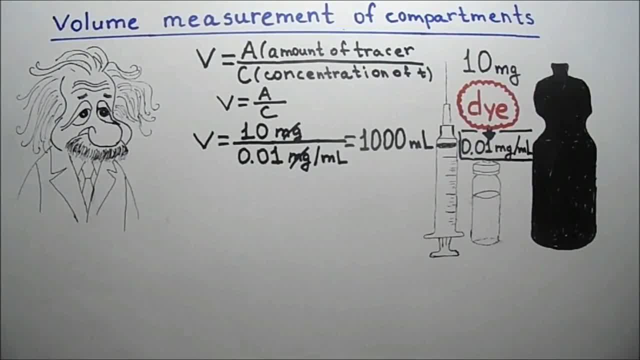 easily measured, well distributed within the compartment and not rapidly metabolized or removed from that compartment. Let me draw here a graph. like in our previous videos, This graph is representing the whole fluid of the patient. Here I'll write intracellular fluid, here the extracellular fluid, which is divided into a iliisticial fluid and plasma. 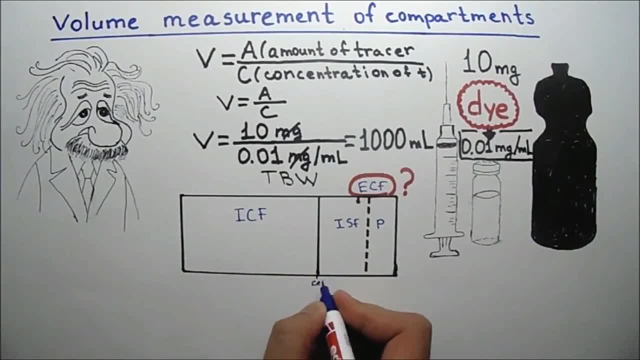 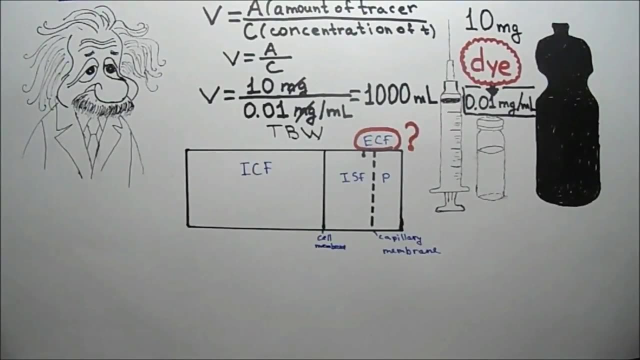 And here I'll write cell membrane and the capillary membrane. Well now, our main goal is to figure out the volume of the extracellular compartment. The wall column of extracellular fluid can be estimated using any of several substances that disperse in the plasma. 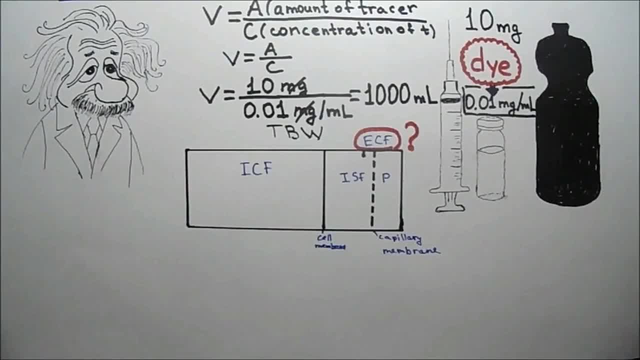 and the intestinal fluid but do not reductively carry it. The problem that my operations shows now is a result of capable do not readily permeate the cell membrane. In other words, these tracers should freely pass through the capillary membrane but not. 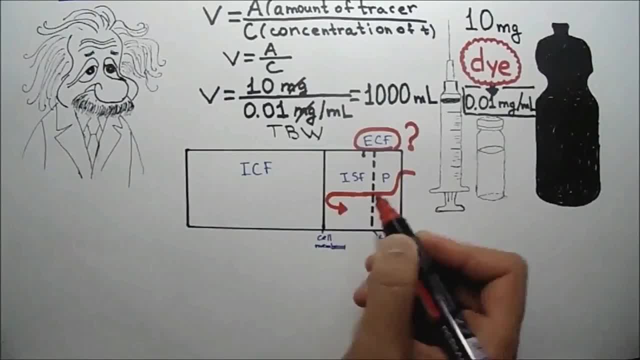 through the cell membrane. The cell membrane should not allow it to move into the cells. This tracer would be well distributed only in the extracellular compartment. Well, inulin, mannitol, sodium and sucrose exactly have these properties. These tracers can pass through the capillary wall, but they cannot permeate the cell membrane. 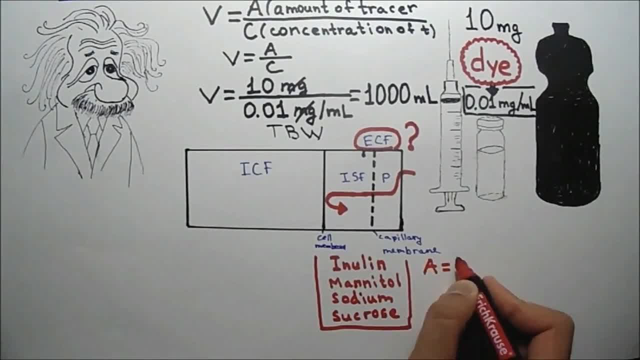 Let's suppose we have injected 300 mg of any above-mentioned tracers intravenously to this patient. Some time after that we have taken a blood and found that concentration of the tracer that we have injected is 0.02 mg per mL of blood. 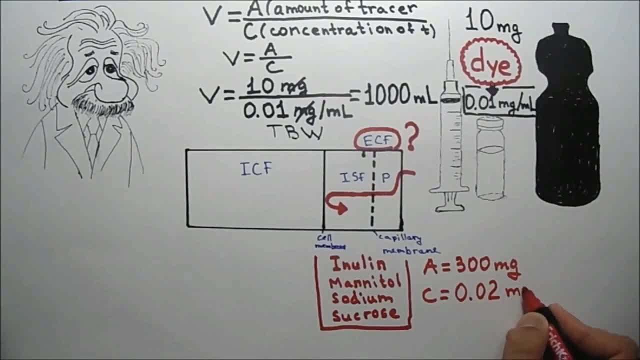 I would not say that these tracers would be distributed in these proportions. It's just an example. To make this concept clearer to you, we have to put these numbers to the formula and estimate the extracellular fluid compartment. So 300 divided by 0.02 equals 15,000 mL, in other words 15 liters. 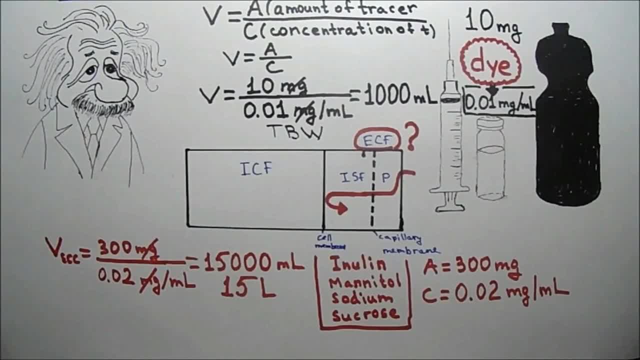 So we can do the same thing: to figure out the volume of other compartments. To estimate the plasma, we can take an albumin, because albumin is a protein which cannot leak out of the capillary. You can find this in the link in the description. 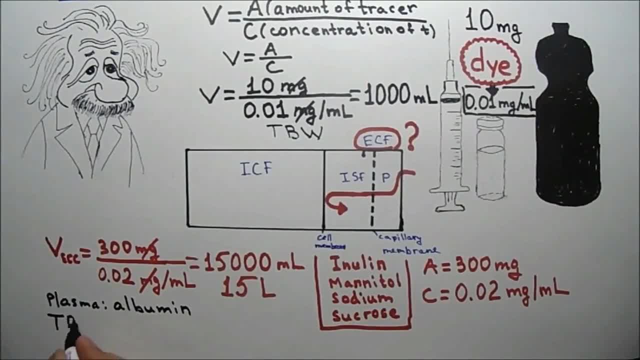 Thanks for watching the video. See you in the next video. Bye. So for calculating total body water, we can use tritiated water or urea, because these two traces can freely pass through all biological membranes. It's very important to note that the interstitial fluid volume cannot be measured directly, but it can be calculated by using this formula. 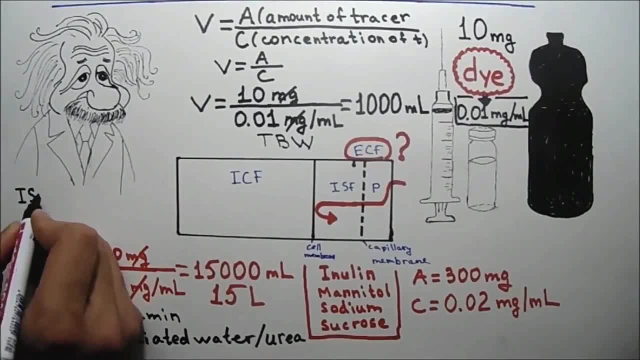 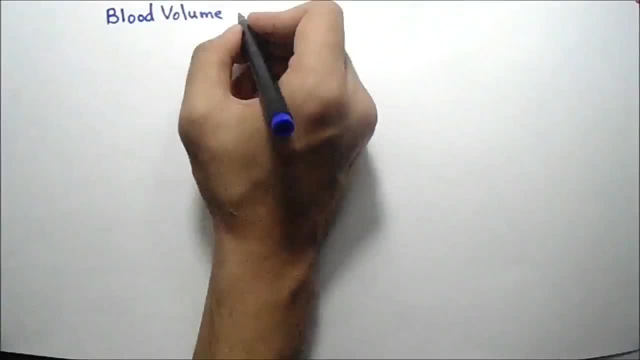 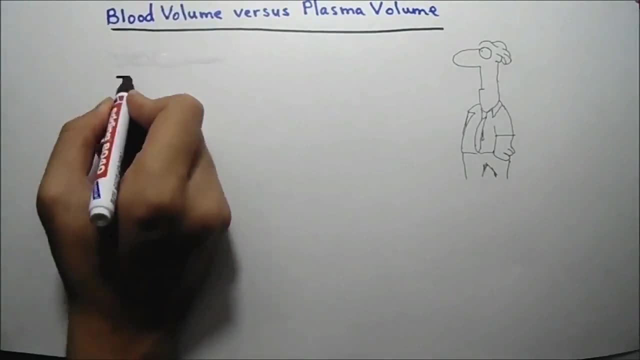 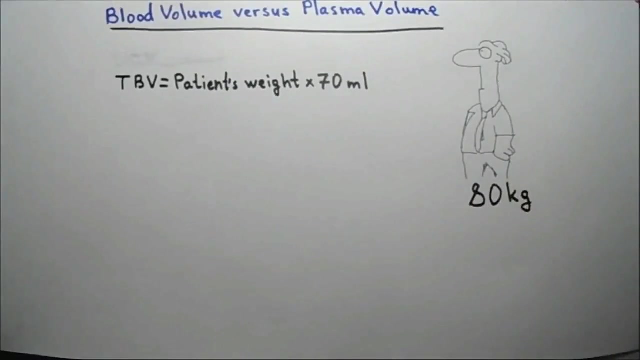 Interstitial fluid volume equals extracellular fluid volume minus plasma volume. Now the second part of our video will be about measurement of blood volume. The total blood volume equals the patient's weight multiplied by 70 milliliters. So if a person weighs 80 kilograms, 80 multiplied by 70 milliliters is equal to 5600 milliliters. 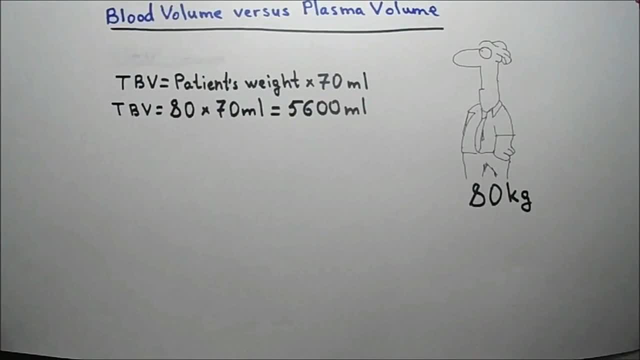 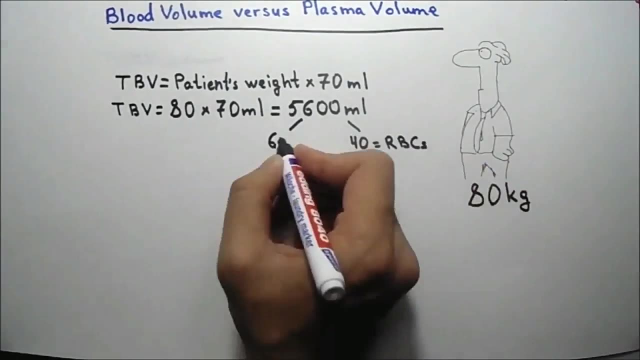 So we got 5600 milliliters And you know exactly well that 40% of this blood is red blood cells And 60% would be the plasma volume right. In other words, hematocrit is 40% in a normal adult person. 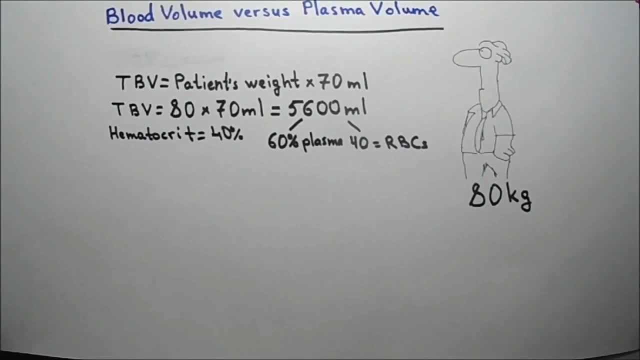 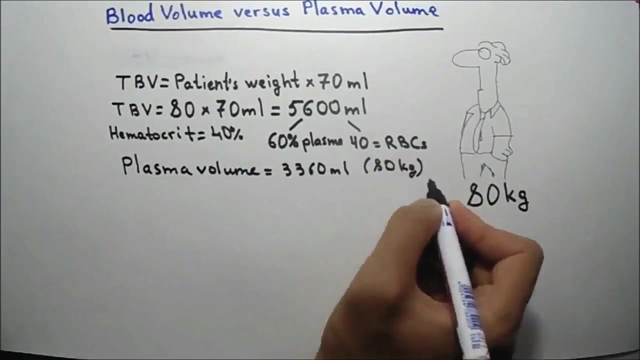 So 60% of these 5600 milliliters will be 3360 milliliters. In other words, plasma volume in an average person weighing 80 kilograms is equal to 3360 milliliters. Now the blood volume can also be calculated. 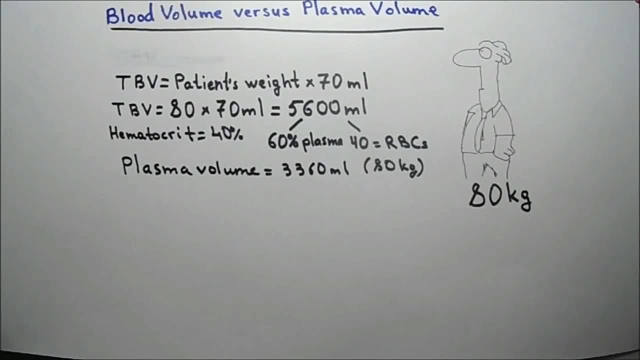 If one knows the hematocrit, Let me assume that you have been given the patient's hematocrit and told to count total blood volume of the patient. If you know the patient's hematocrit, you can calculate the total blood volume using this formula. 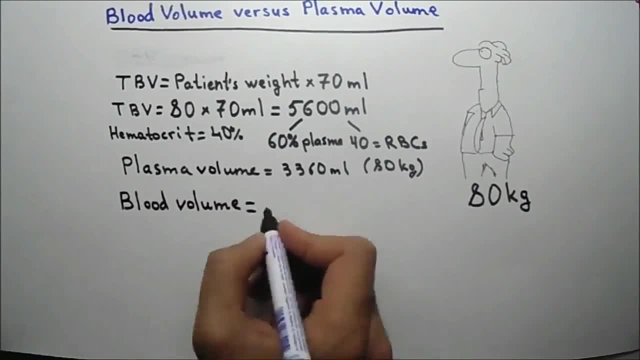 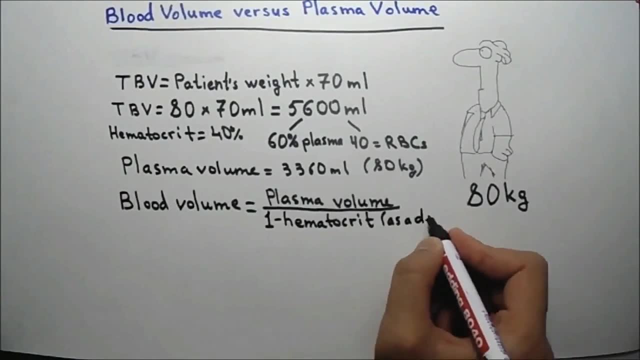 Blood volume equals plasma volume dividing by 1 minus hematocrit- Hematocrit as a decimal. Let's suppose that the patient's hematocrit is 50%, And here we have a patient's hematocrit And he weighs 80 kilograms.